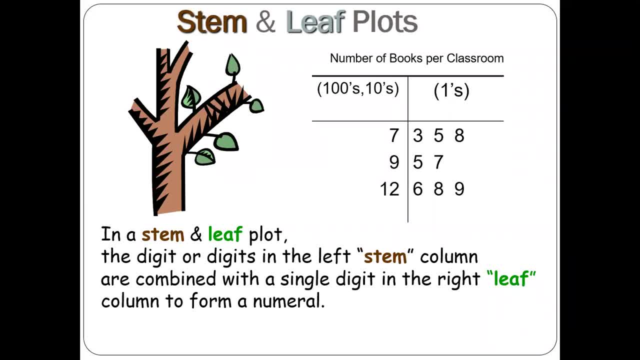 with the digit in the right, that is the leaf column, to form a new mirror. Now, in the stem column we have 7, the leaf column, we have 3,, 5 and 8.. So here we will take 7 and combine with 3, and we will have 73,, 75 and 78. 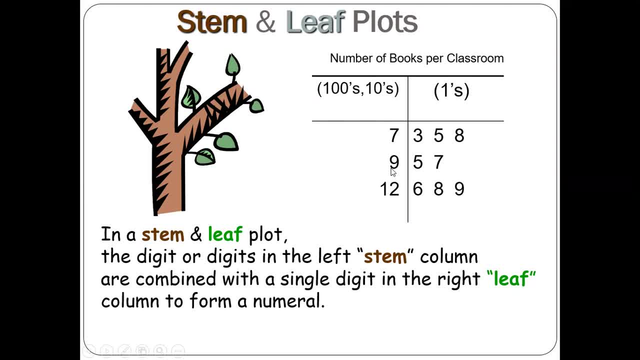 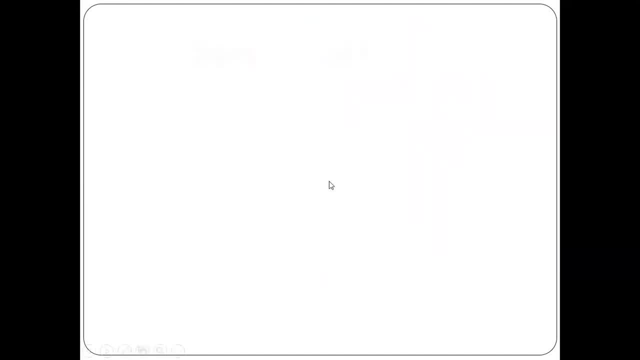 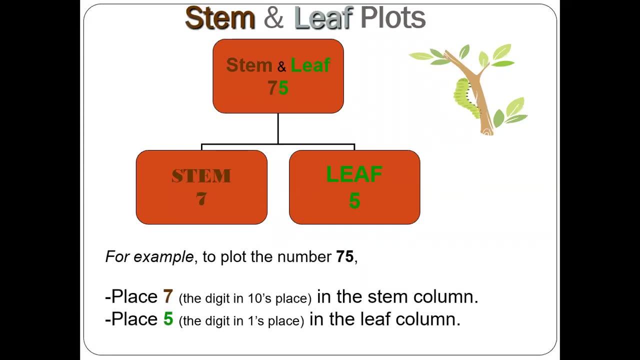 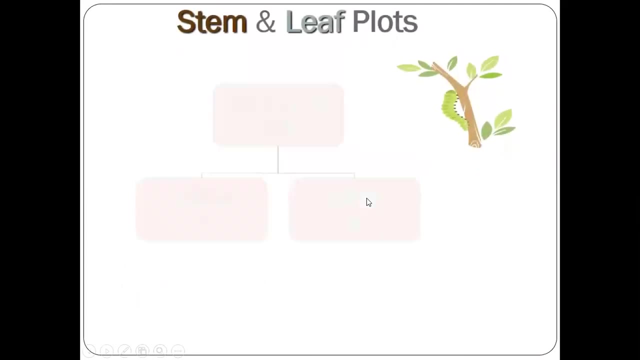 So those are the digits that we are going to obtain there Same year, 1978.. 95,, 97.. More around 26,, 128 and 129.. So if we have 75,, 7 becomes the stem and 5 becomes the leaf. 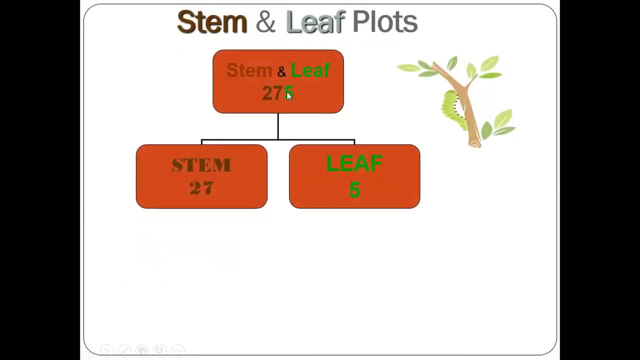 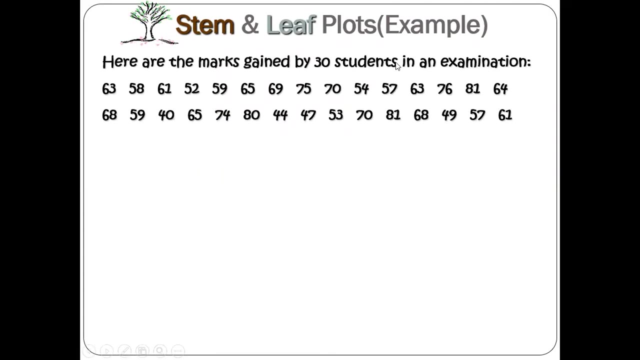 In case we have a three digit number, 275,, 27 becomes the stem And the three digit number 28 becomes the leaf. So let's take this example. Here are some marks gained by 20 students in an examination. So we start by taking the first digits of all these numbers, without repetition. 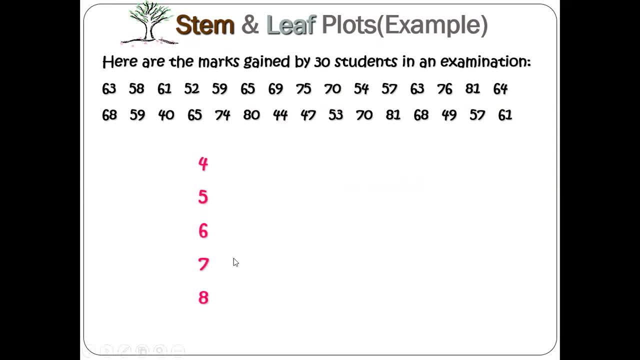 Now we start with the first digit, which is four. The first number here that starts with four is 40. So we'll take that, we take 40, we are remaining zero, right zero. there, at the level of the lift, we are 44, so right, 4. 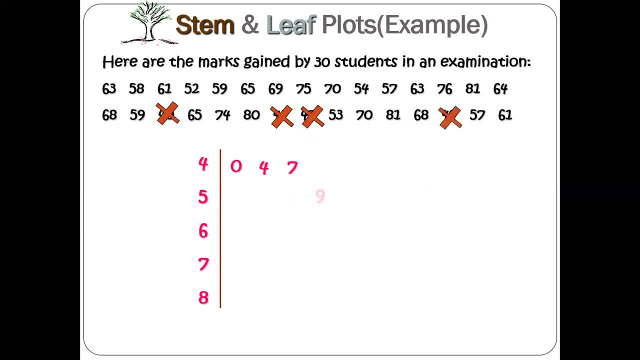 47, 7, 49, right, 9.. so do same for all the remaining digits. so for five, this is what we are going to have. for six, we'll have these seven days and eight days, using the same procedure that we have used for before, and from here we obtain our stem and leaf plots. thanks for watching. 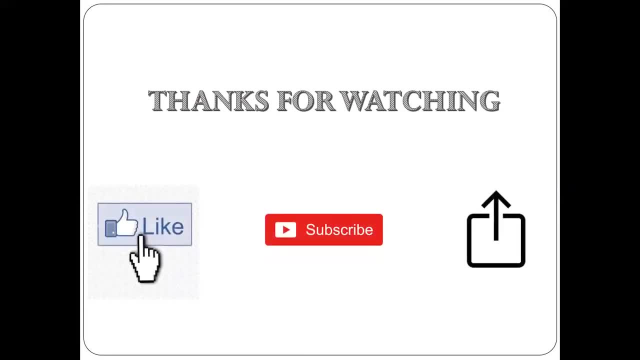 and don't forget to like, subscribe and share.